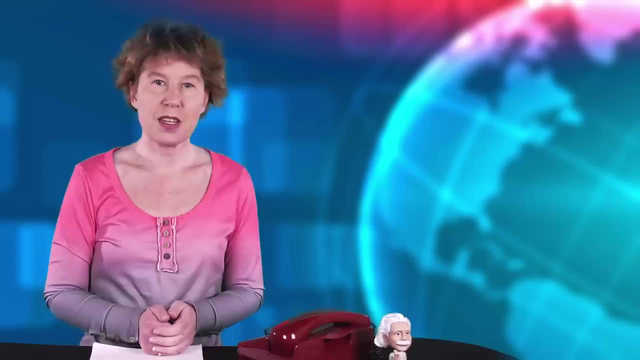 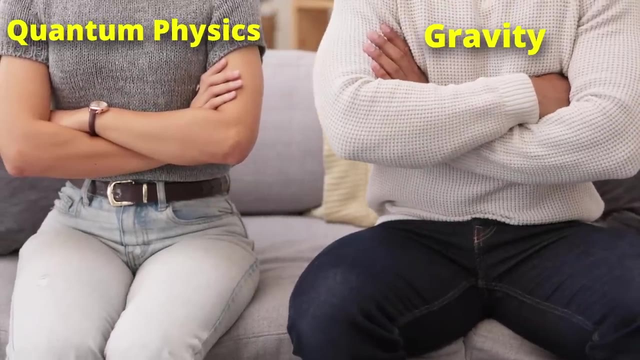 matter and dark energy. Let's have a look. This video comes with a quiz that lets you check how much you remember. Quantum physics and gravity don't get along with each other very well. Quantum physics is what we call a non-deterministic theory. It has a random element. 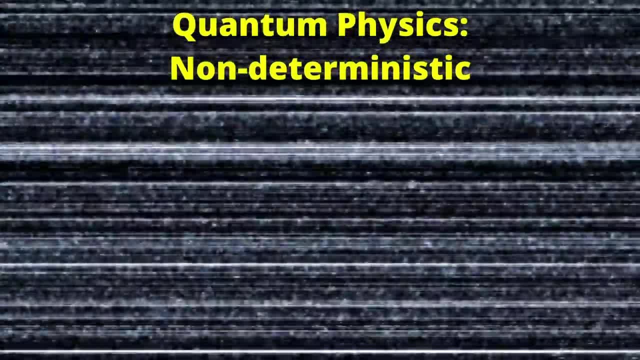 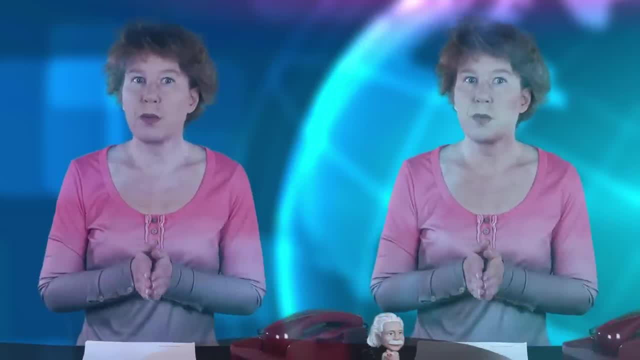 it has built-in uncertainty and it sets limits to what you can know and do. We often say that quantum particles can be in two places at once, but really what the math says is that it doesn't make sense. It's just that you can't know what's going on between them. So let's have a look. This video comes with a quiz that lets you check how much you remember. Quantum physics and gravity don't get along with each other very well. Quantum physics is what we call a non-deterministic theory. It has a random element. it sets limits to what you can know and do. We often say that. 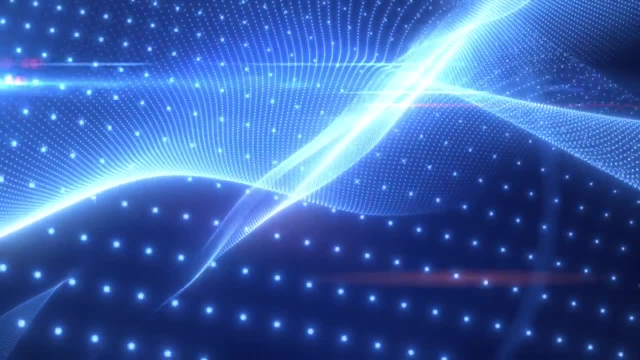 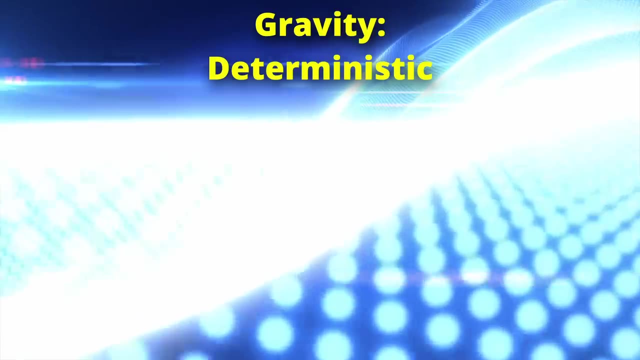 quantum physics is what we call a non-deterministic theory. It sets limits to what you can know and do. Gravity, on the other hand, is described by Einstein's theory of general relativity. It assigns a time and place to everything. It's deterministic. the future follows from the past. 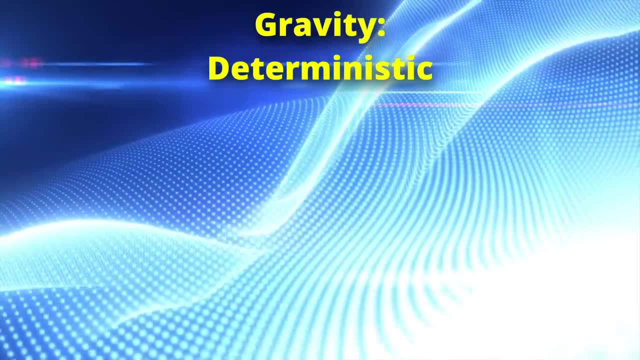 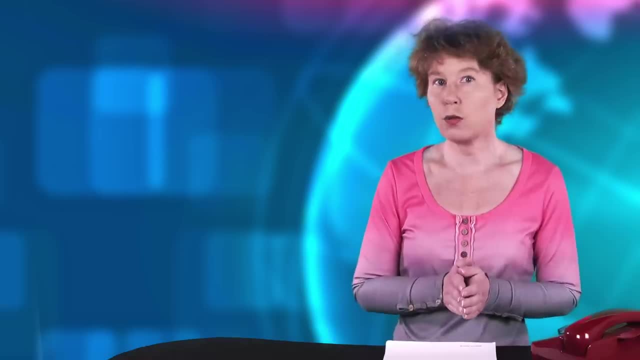 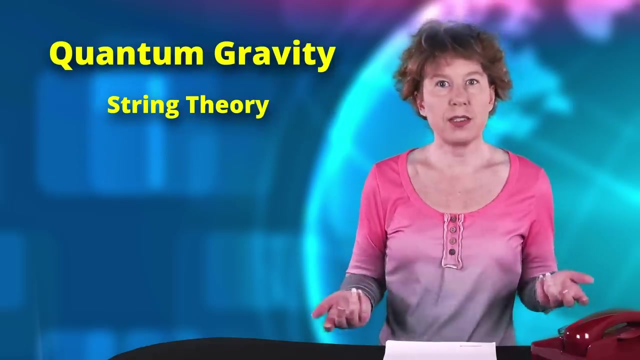 and the only uncertainty it has is that stemming from our own lack of knowledge. There have been many attempts to unify the two and create what's known as a theory of quantum gravity. The best known approaches give quantum properties to gravity gravity and include string theory, loop quantum gravity and asymptotically safe gravity. 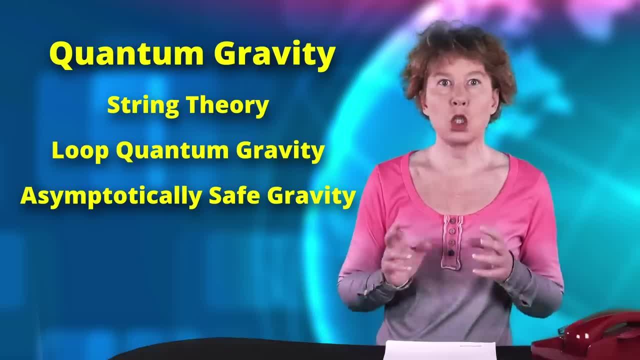 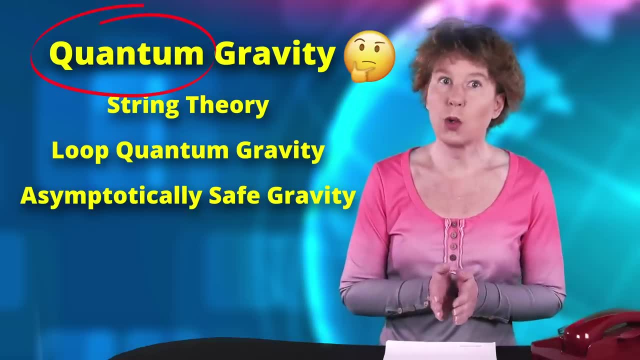 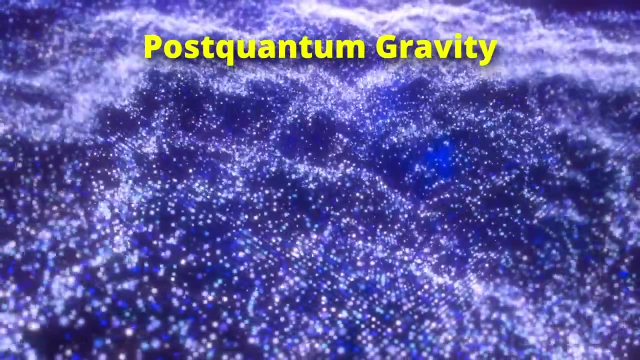 The path less taken is to leave gravity a non-quantum theory or to change something about quantum physics. These ideas have not worked out all that well so far. Oppenheim's new idea, post quantum gravity now, is to combine gravity and quantum physics by giving a random element to gravity. This randomness doesn't come from anything, it's 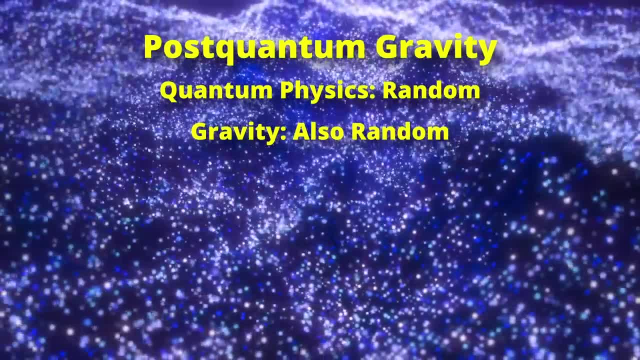 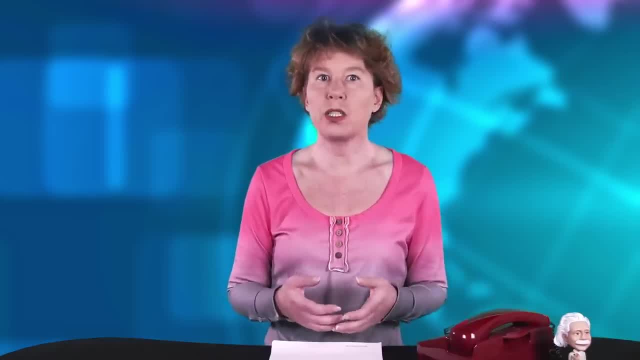 a fundamental ingredient. it's the starting point. This is just like the randomness of quantum mechanics does not come from anything else. it's fundamental, a starting point, just a property of nature. The innovation that Oppenheim brought in now is that he found 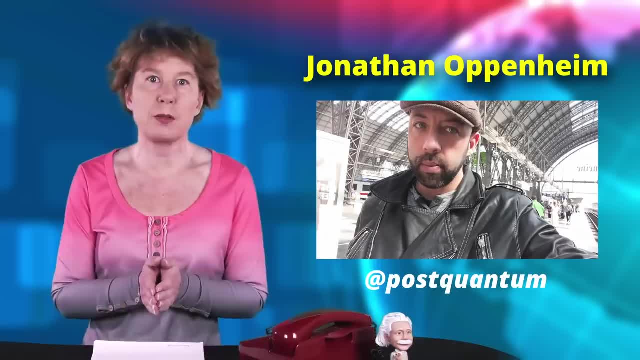 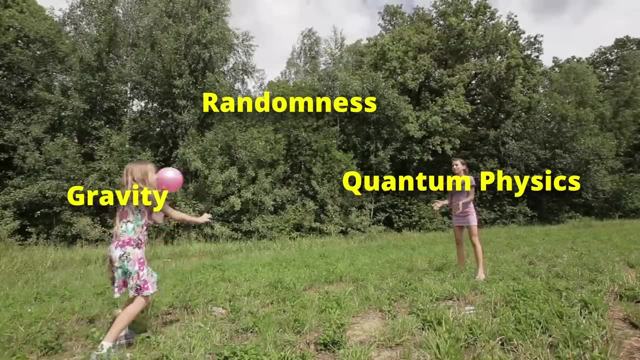 a way to combine the mathematics of both types of randomness into one framework. In this post, he found a way to combine both types of randomness into one framework. In this post-quantum theory, quantum remains non-quantum and particles remain quantum. However, these 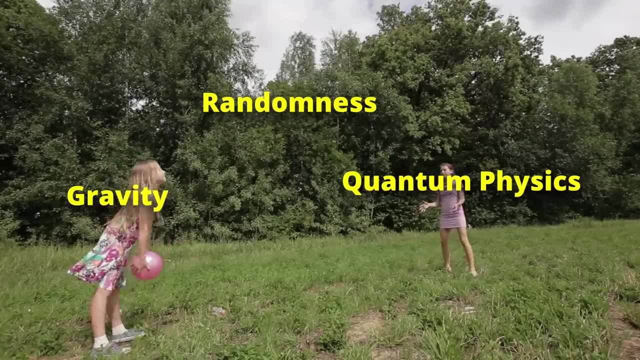 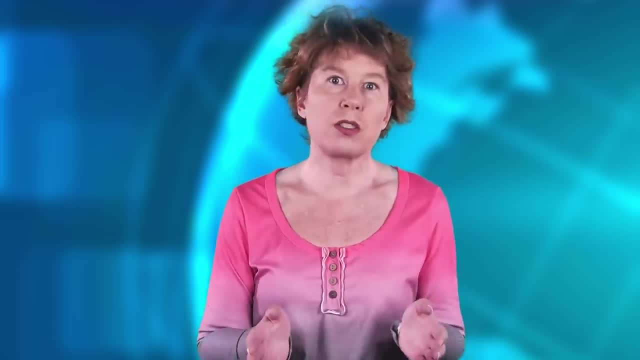 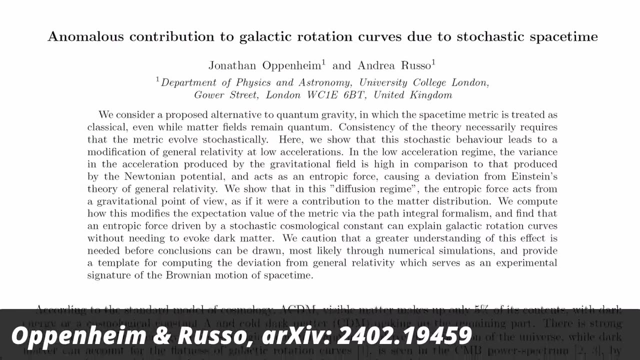 two sectors communicate with each other because particles have gravity and that gravity in return influences the particles. In Oppenheim's theory this works without contradictions because these two randomnesses fit together In the new paper now, Oppenheim and his co-author Rousseau say that this randomness changes the law of gravity under certain circumstances. 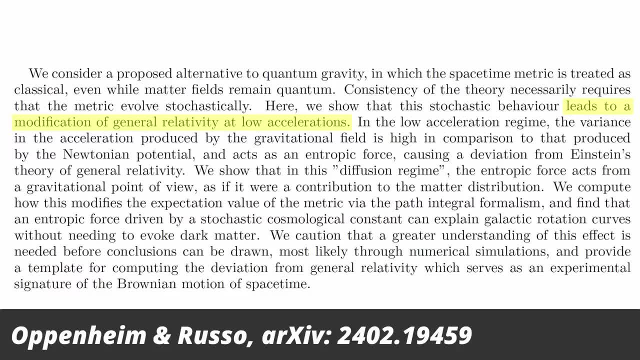 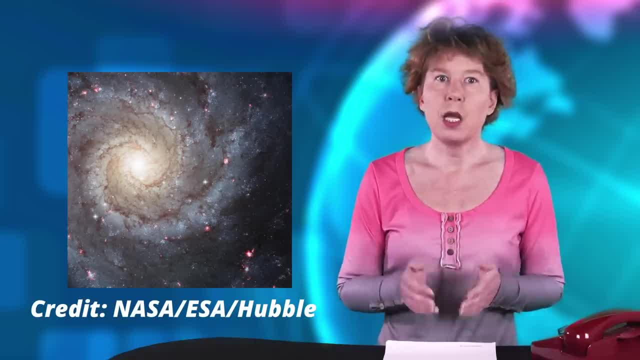 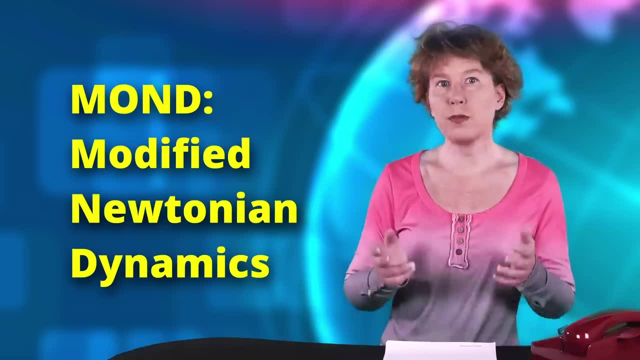 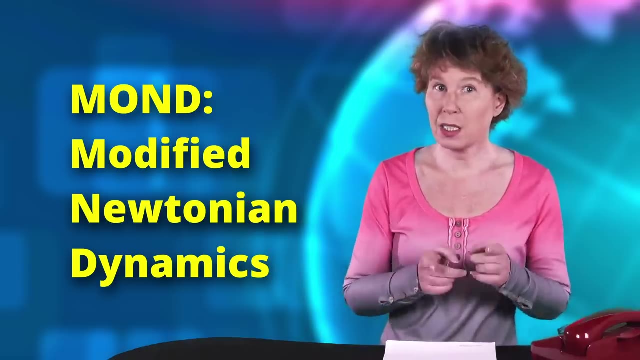 And those circumstances are when the acceleration of an object is very small. If you followed the debate about dark matter, then this'll immediately ring a bell, Because the major competitor of dark matter is a modification of Einstein's gravity, known as Modified Newtonian Dynamics, or MOND for short, And that becomes noticeable- wait for it- at small. 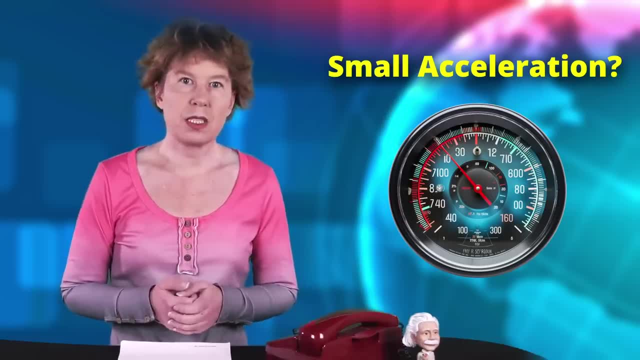 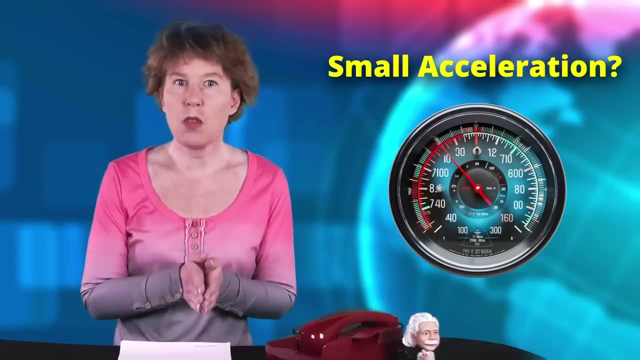 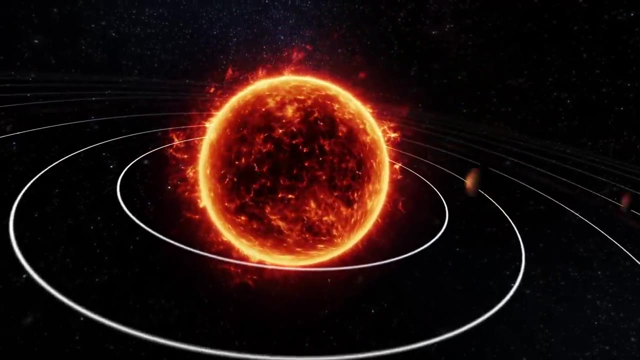 acceleration. The reason this modification at small acceleration can appear as if there was dark matter is that the acceleration on average depends on the strength of gravity. If you are near a planet or a sun, like most of you probably are, then you experience a noticeable pull. 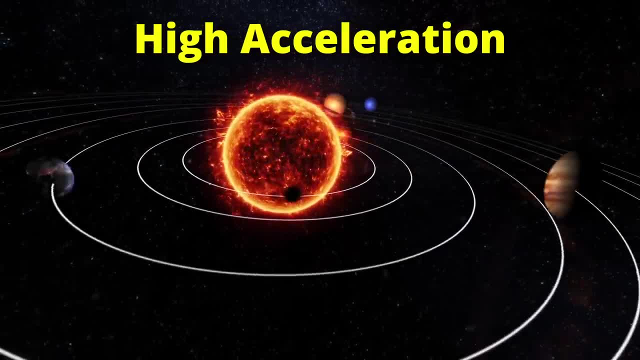 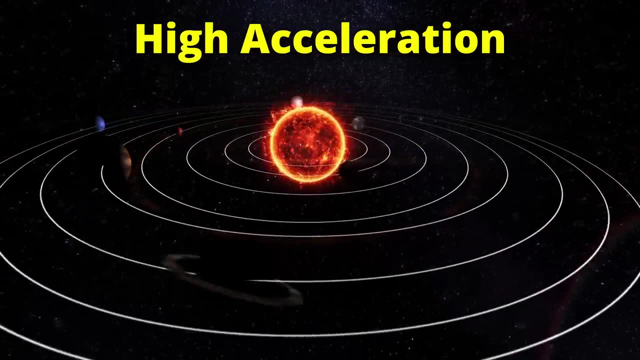 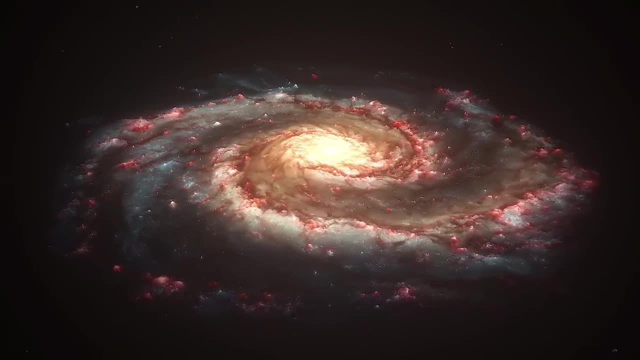 of gravity from those heavy objects. If you interpret that as a force, then that gives rise to an acceleration. The farther away you are from heavy objects, the smaller the acceleration. However, the overall gravitational pull coming from the entire galaxy gets smaller the farther. 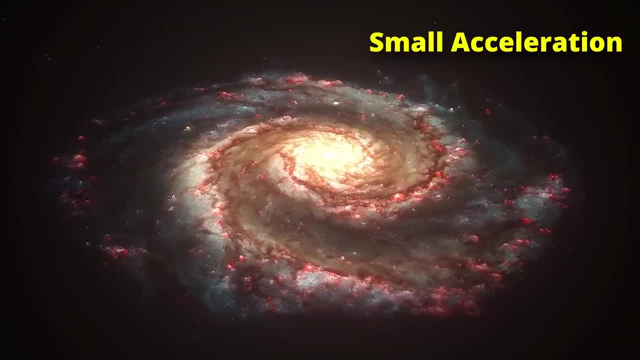 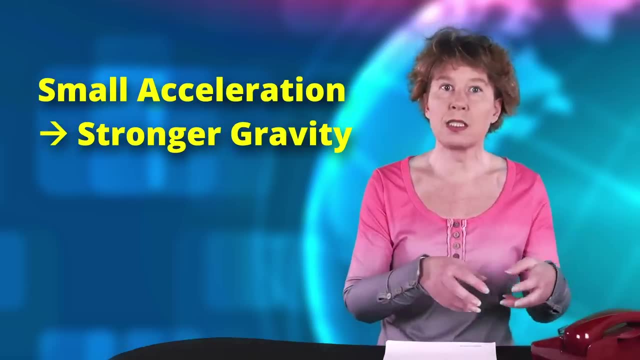 away. you are from the center. This is just because most of the mass of the galaxy sits in the center. It now turns out that if you assume that gravity gets stronger at small acceleration, then that can explain the observations attributed to dark matter in galaxies. This 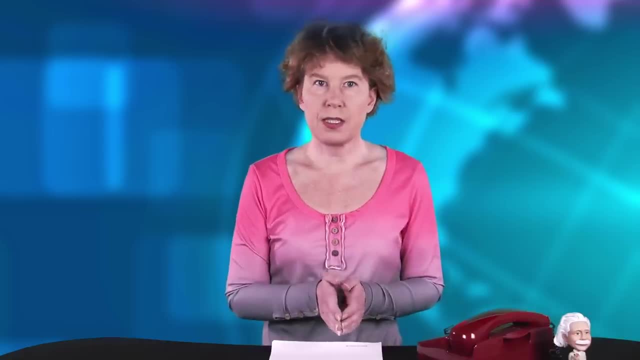 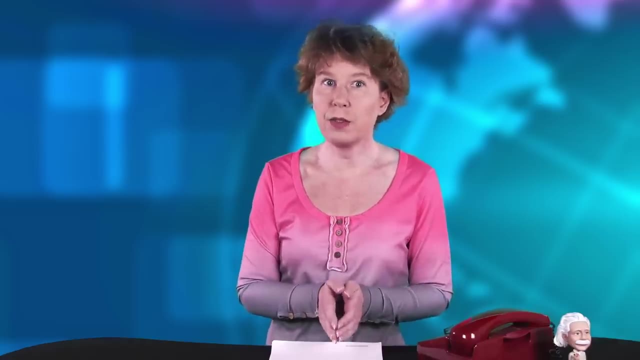 is, in a nutshell, the idea of MOND. Oppenheim now says that when they look at the changes that they get to the law of gravity from this randomness, they see a similar behavior. The smaller the acceleration of an object, the more its affected by the randomness. 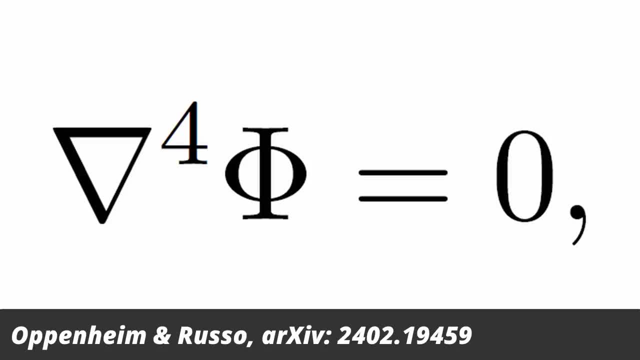 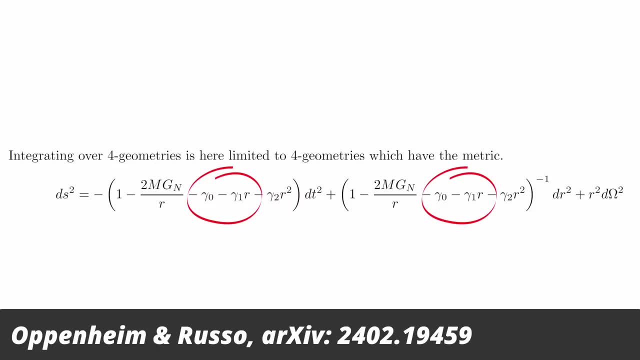 They derive an equation that is similar to Newton's law of gravity for the Newtonian potential, and then they have some unusual contributions. they show that these extra contributions seem to be similar to those of modified Newtonian dynamics, which is dark matter's competitor. 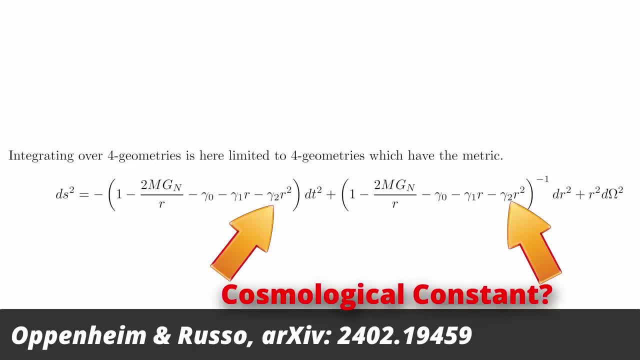 Yet encyclopedia with full principio from Skevyn Smith created this equation called Newtonian law of gravity. according to Newtonian oczywiście math, It probably means that N постоян is to that they say, looks like dark energy. On Twitter, Oppenheim writes: 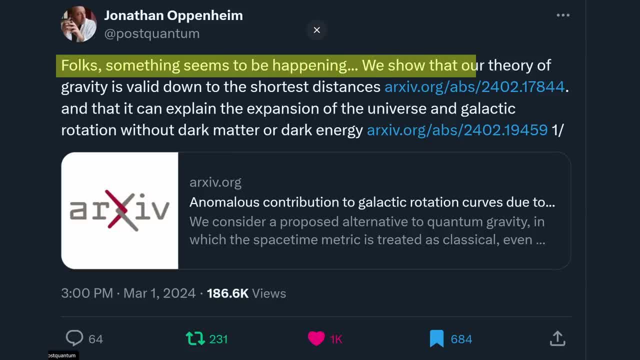 Folks, something seems to be happening. We show that our theory of gravity can explain the expansion of the universe and galactic rotation without dark matter or dark energy. Okay, but you didn't come to hear what the authors say about their own paper. Let me guess. 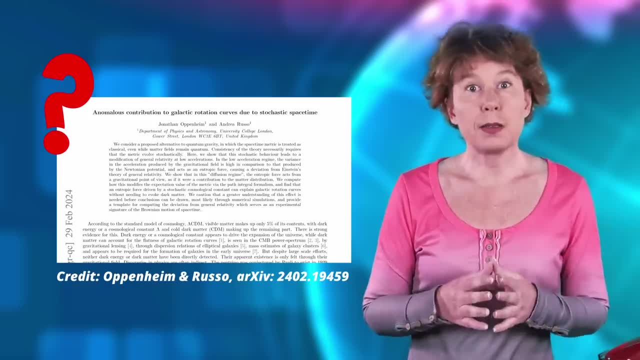 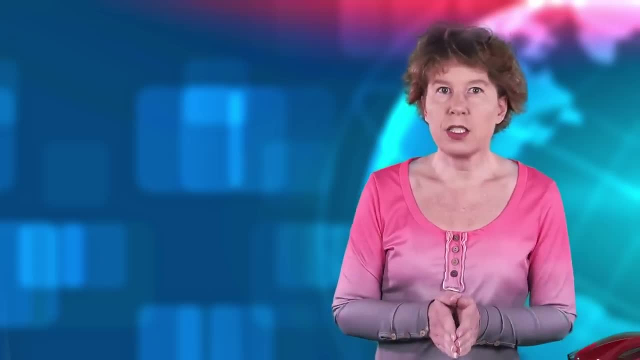 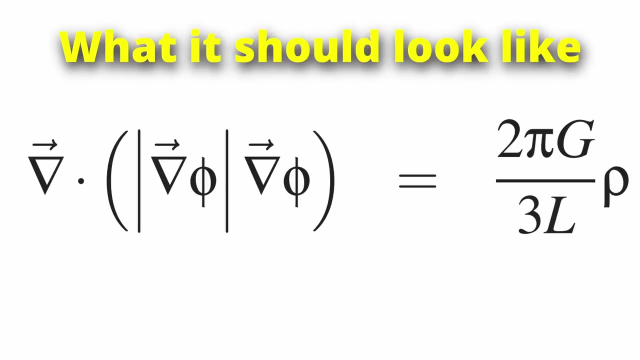 you came to hear what I say. Alright, I actually don't like doing this, but here we go. I think it won't work. The reason is that the equation they have is linear in the Newtonian potential. To make modified gravity work, you need an equation that's non-linear in the potential. 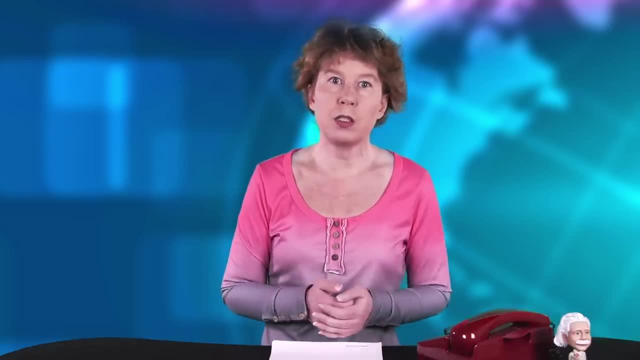 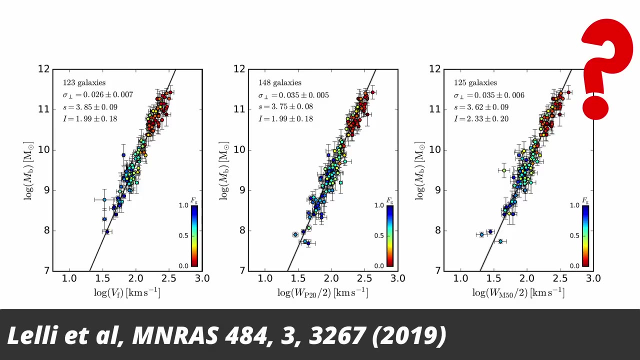 I haven't had time to think about it much, but I expect that if you look at the scaling of the asymptotic velocity with the mass of the galaxies, it won't come out correctly. The only differential equations that get this right have a rather peculiar non-linear form with a 3 over 2 exponent. 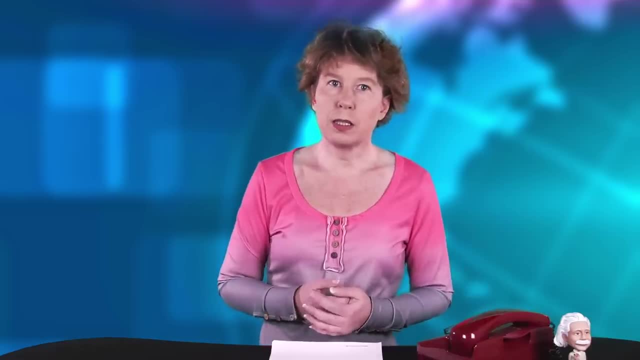 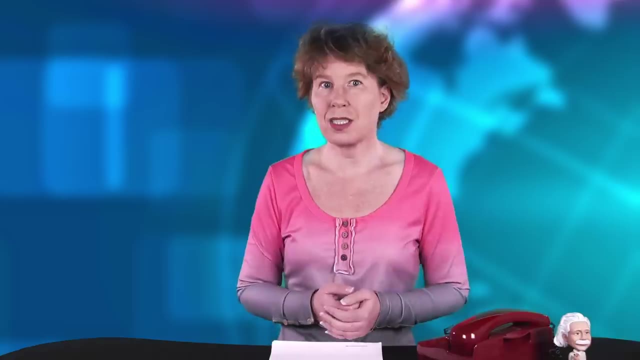 So yeah, I kind of wish it'd work, but I don't think it will. But you know, I'm just an old grumpy woman who thinks she's seen it all before, so maybe it turns out that what I just said in front of some 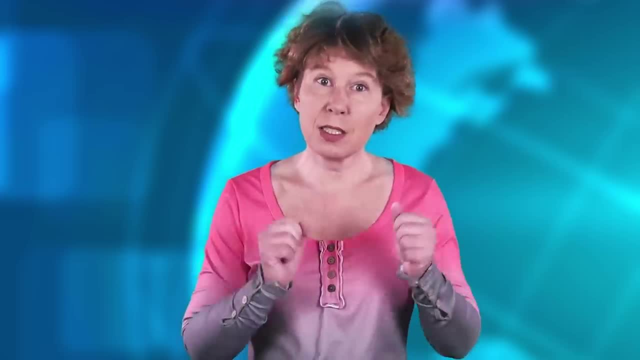 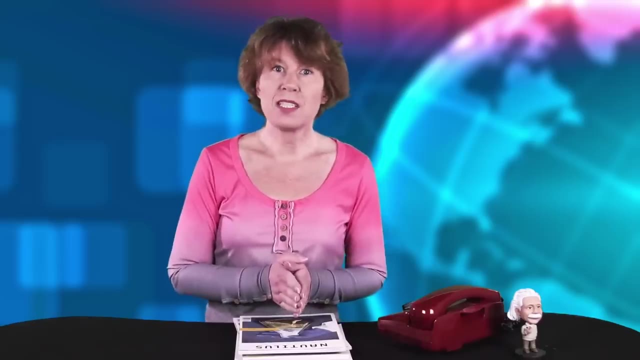 hundred thousand people was complete nonsense, And if that turns out to be so, you don't want to miss my public embarrassment, so stay tuned. If you'd like to learn more about recent scientific developments, I recommend you have a look at Nautilus magazine. Nautilus is a science magazine. 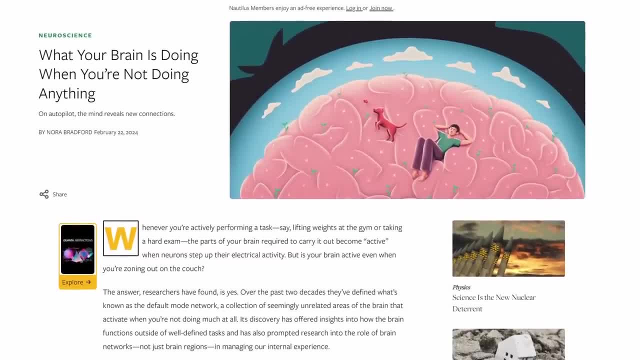 that keeps you up to date on the most relevant topics in the world, And if you'd like to learn more about the topics that are being discussed today, you should definitely visit the site of Nautilus. They frequently have scientists writing for them. who'll tell you the inside. 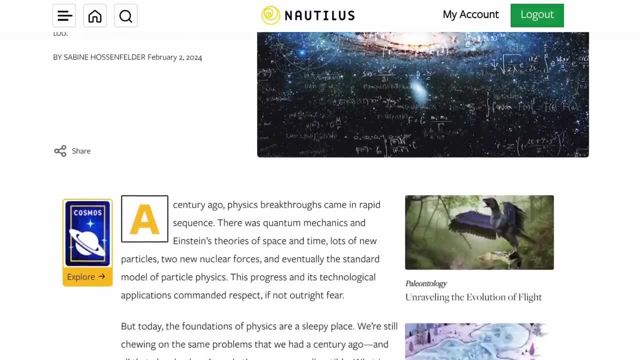 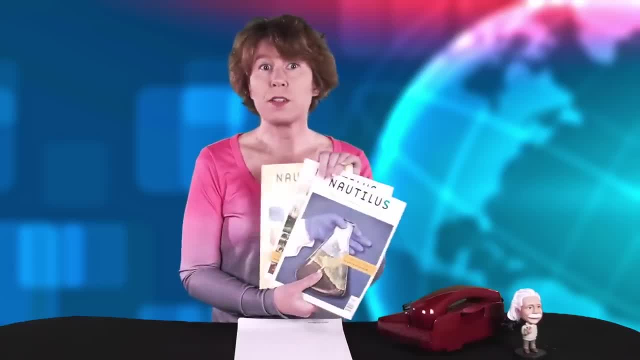 stories. I've written a few contributions for them myself, most recently about John Oppenheim's theory of post-quantum gravity. Nautilus comes with a digital and a print version and it's just a pleasure to read. They really put a lot of effort into writing. 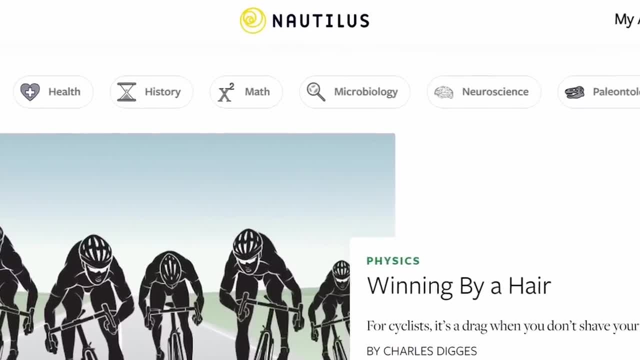 and the graphic design is top. What I particularly like about Nautilus is that they cover all areas of science, from astronomy to economics, history, engineering and astronomy. All of this really helps you to get the hang of the topic, But if you're not sure what you're looking for, you don't.